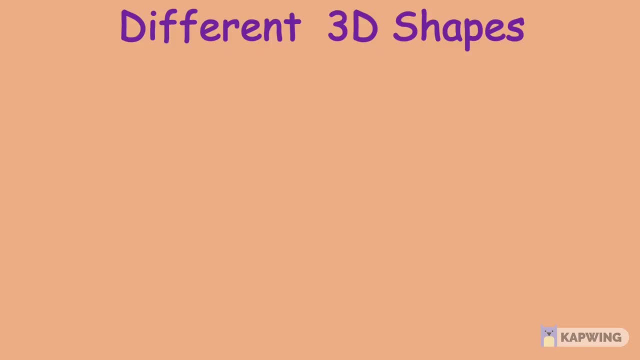 This is a good example for a 3D cone shape, And our next 3D shape is a cylinder. A cylinder has got a circle on the top, a circle on the bottom and smooth all around. Example we have got is a can. Here you can see. 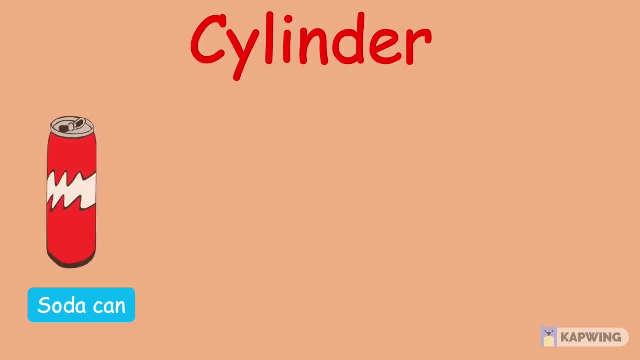 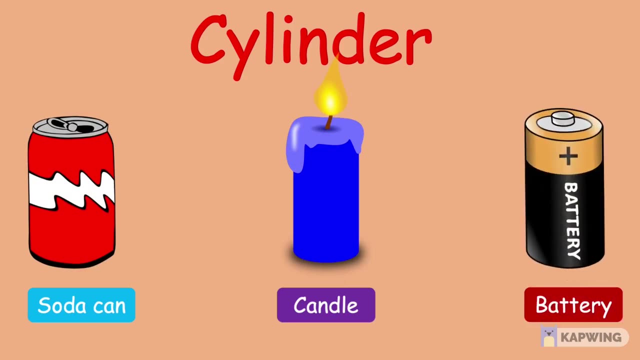 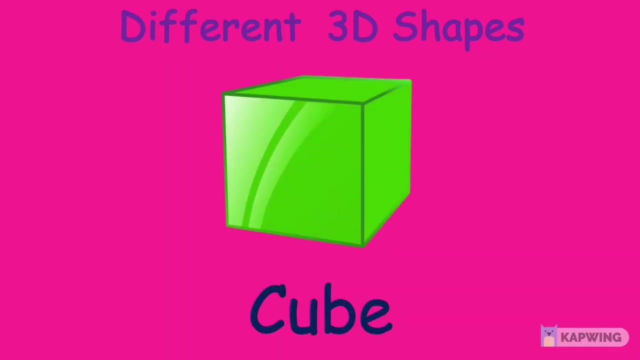 it has a circle on the top, a circle on the bottom and smooth all around. In the same way we can take candle and battery as an example for cylinder 3d shapes. this shape is a cube. a cube has six sides, or faces that are all squares. here you can see two dice in the shape of a cube. 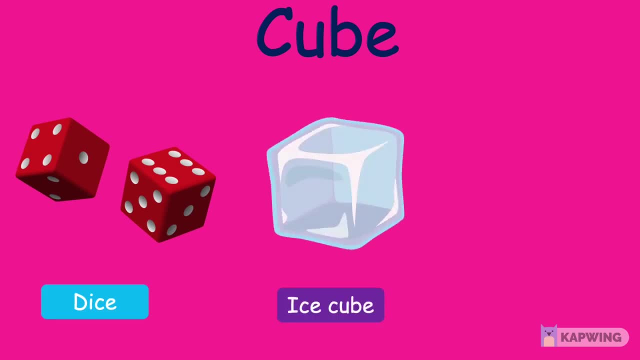 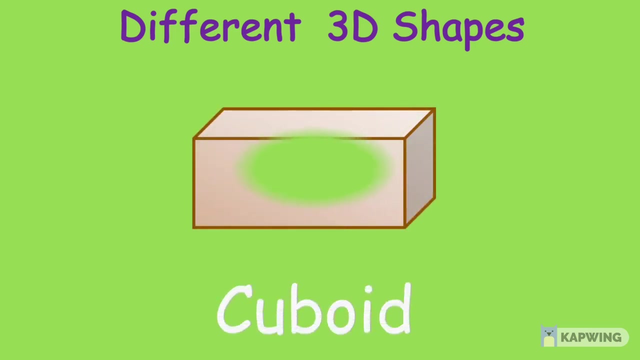 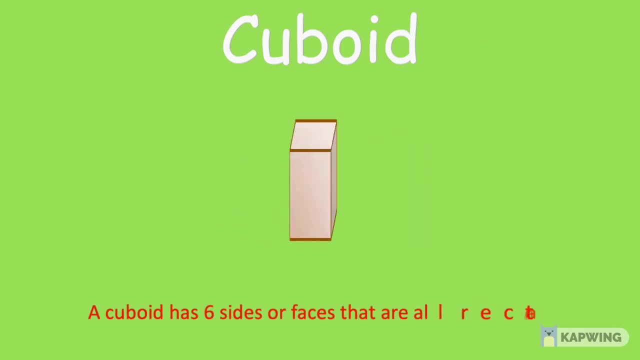 then we can find an ice cube which has six sides or faces and they are all squares. and we have got four rubik cube and all of them have got the same cube shape. and lastly we have is a cuboid shape. a cuboid has six sides or faces that are all rectangles. here we have a carton box. 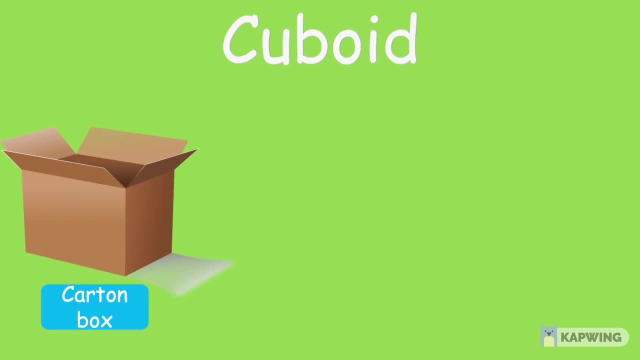 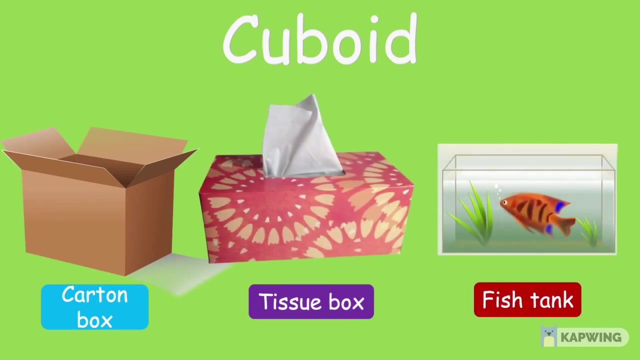 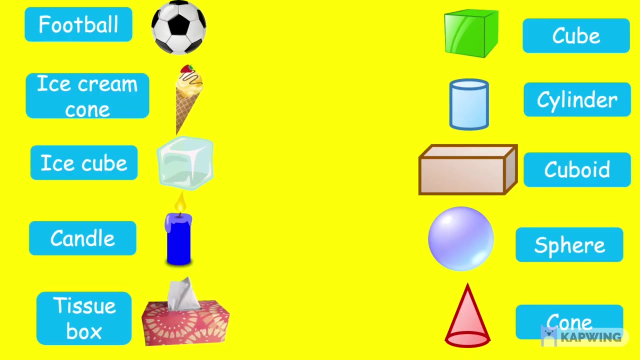 with six sides or faces. they are all rectangles. we also have a tissue box in the shape of a cuboid, and a fish tank is also a good example for a cuboid. so, children, let's recall by matching all the objects with the following 3d shapes. so what is the shape of the football here? yes, a football. 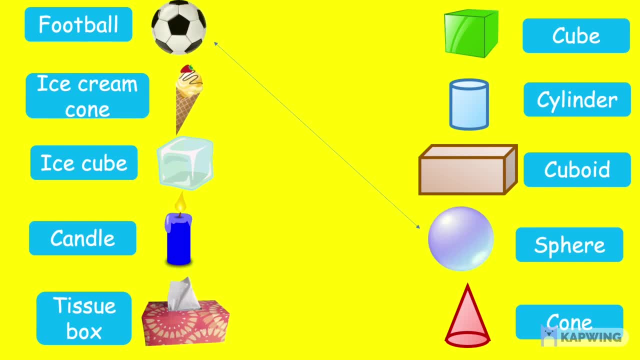 is the shape of a sphere. what about an ice cream cone? an ice cream cone is in the shape of a 3d cone, an ice cube. what shape does it belong to? yes, it belongs to a cube- 3d shape. next we have is a candle. candle belongs to a cylinder- 3d shape, and we can take this tissue box as an example for a.